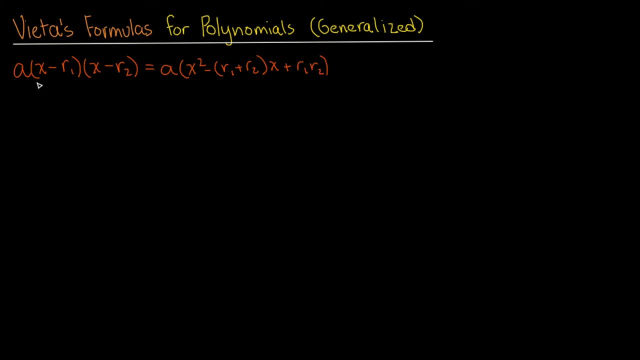 In the previous video we looked at how Viettas formulas could be used for quadratics and how they can provide useful information, such as the sum of the roots or the product of the roots, But it does raise an interesting question of what happens when we increase the size of the polynomial. 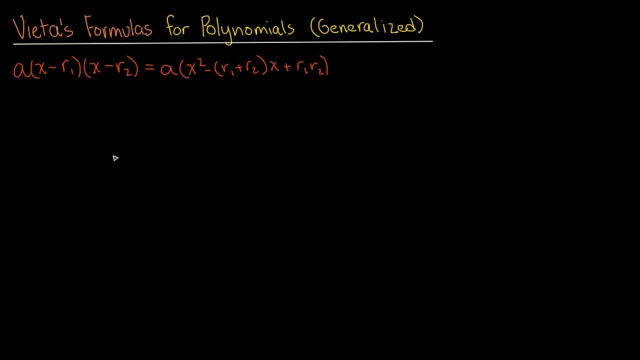 What if the polynomial is a third degree polynomial or a fourth degree polynomial? So let's look at that. It's an interesting question and the first step when trying to figure out something like this is probably to experiment around. So we expanded two binomials in the previous video and I changed the roots to R1 and R2, as it will hopefully make things clearer later on in the video. 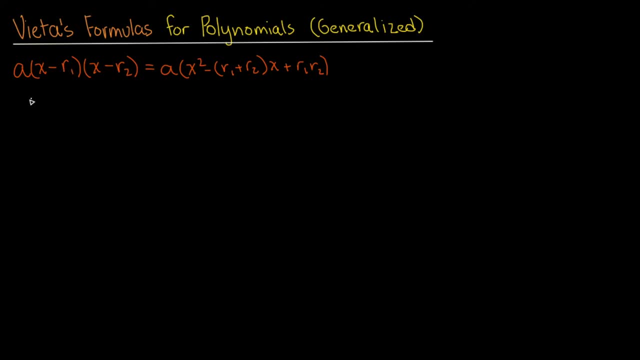 But the first step would probably be: well, let's go to three binomials, Let's see what happens, What happens when we expand three binomials. So we'll have the same ones as above, but we'll also add an extra X minus R3.. 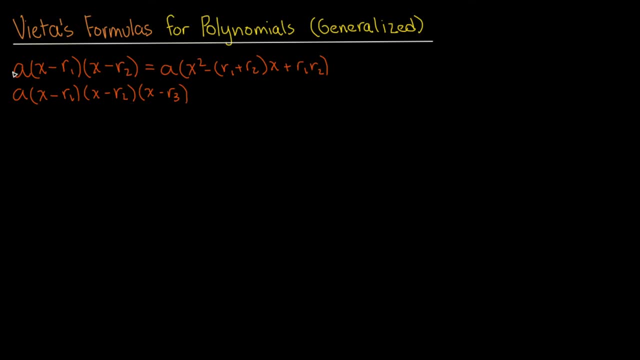 And, as you can see, the first part is equivalent to the part over here, So we can just write down what we wrote before. Now we have to, of course, multiply our extra binomial that we have left. The way I like to expand polynomials that are multiplied together is write it in an order based on the last polynomial. 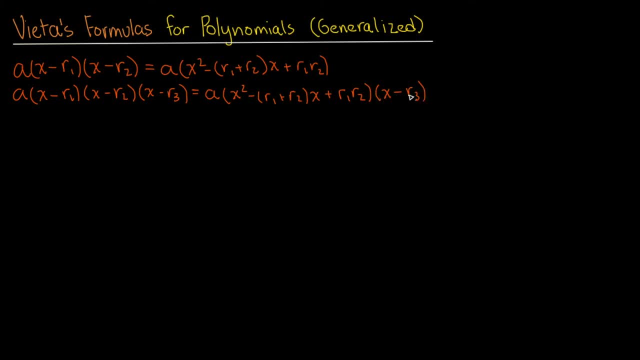 So, for example, when I'm multiplying this X minus R3 to this quantity over here, I'll first multiply it with X and write that down, and then multiply it by R3 and write that down below that. So let's actually do that. 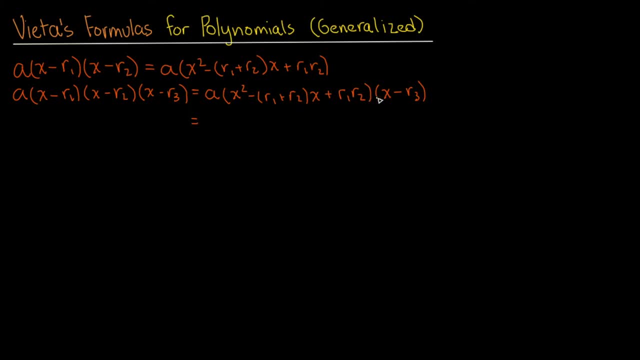 We're going to set this equal to, And we'll still keep the A on the outside. So I'm going to- I'm just going to write a, A times all of this on the outside. Let's expand the inside now. So X times X squared would be equal to X cubed. 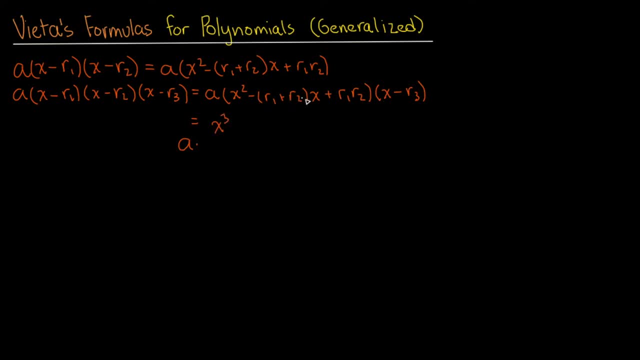 X times negative. R1 plus R2X would just be negative- R1 plus R2.. X squared. And then we have the plus R1, R2, X and I'll expand the R3 part of it. So, since it's the, when we multiply R3 to X squared, it's going to be negative R3- X squared. 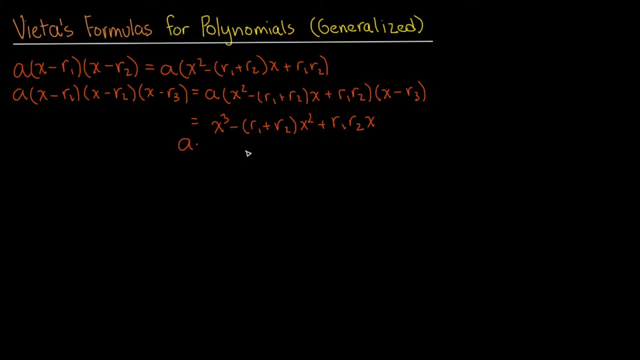 I'll put it below the X squared term over here. So we have negative R3, X squared. And then we have, when we multiply it here, we have a negative times a negative, And then finally we multiply it by the last one. 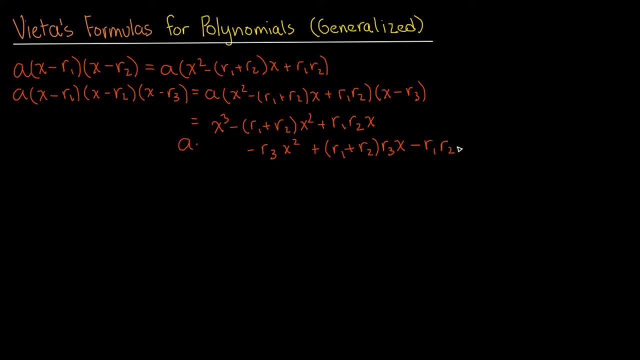 So it's negative R1, R2, R3.. So let's look at, let's look at what happens when we add this entire thing. Let's keep this A on the outside and we have our X cubed. Now, when we add this negative R3, X squared to this term. 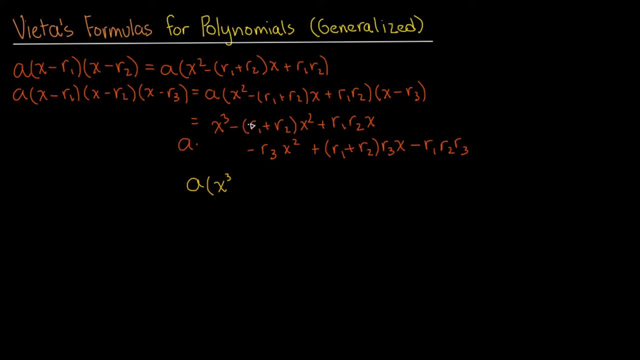 over here will be the negative we can take outside, as before. So we'll be left with minus R1 plus R2 plus R3 times X squared. And now for this one, when we, when we multiply R3 to each of these, then we'll be left with plus. 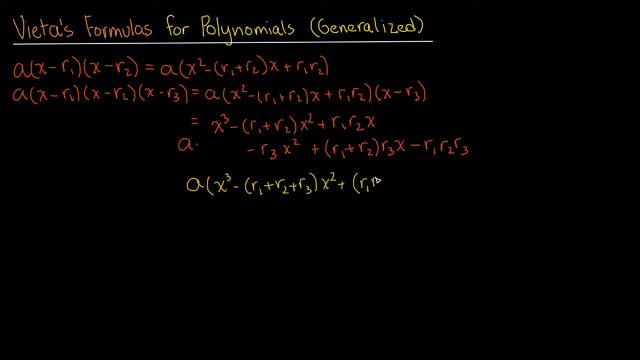 R1, R2 from the first one over here, and then we'll have an R1, R3 when we distribute the R3 plus R2, R3, which is this one over here, And we'll have to multiply that to X. 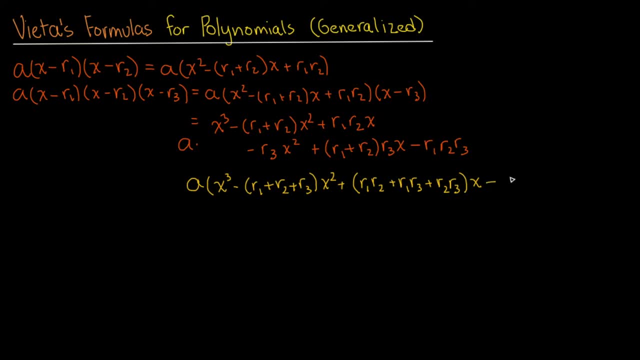 Finally, we have our 3 R1, R2, R3 over here. So that's interesting. Our original roots were R1, R2, R3.. So this, still the second coefficient of our polynomial, is still A times the negative of the sum of the roots. 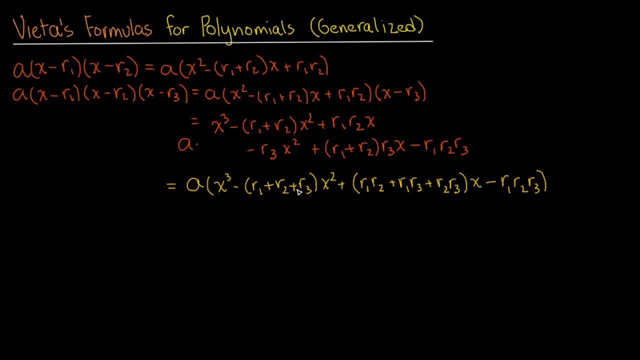 which is the same as what we saw in the quadratic, in the quadratics video about Vieta's form. So but there is a new thing over here: There's still the product of the roots at the end over here, except it's negative. 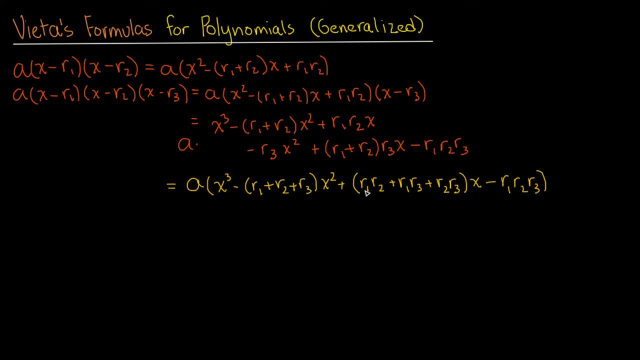 which is something to take note of. But there is something new here. We have a looks kind of like a permutation of the values of the roots. So we have: first we multiply the R1 times R2,, then we multiply the R1 times R3.. 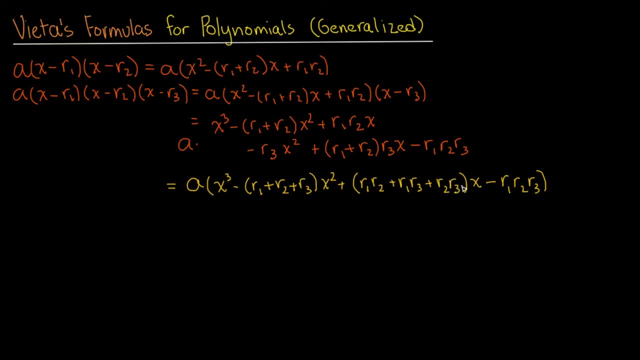 Then we finally do the combination- that hasn't happened- R2, R3. And so we should start to get some idea here of what is going on, And that is the basis for how Vieta's formulas actually works. So first we have the R1, R2, R3. 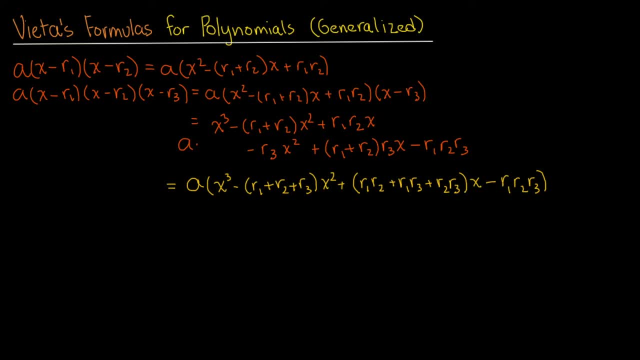 First of all, let me write out the standard form of a cubic. just to compare: Ax cubed plus Bx squared plus Cx plus D, And so when we have Ax cubed that is accurate, We see an A times an x cubed. 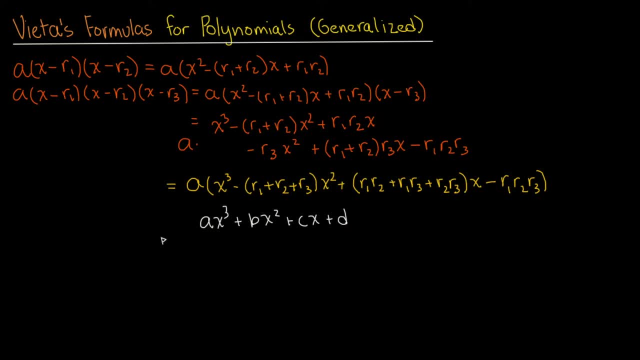 But what we're seeing here is that B. So we can actually write these down for cubics. So this is the- you can say the cubic, the Vieta's formulas for cubics. So we can say that B is equal to A times the negative of the sum of the roots. 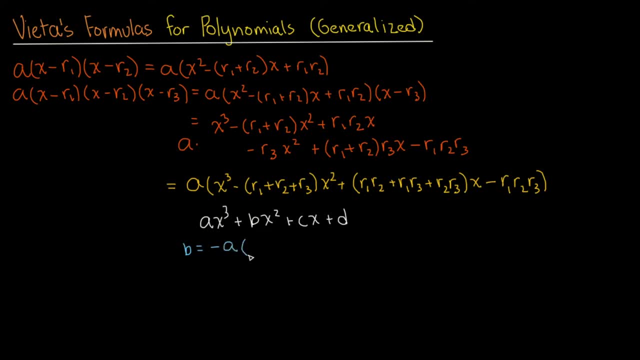 So we can keep the negative A times R1 plus R2 plus R3. So that's negative A times the sum of the roots, And we can- we can divide by negative A on both sides And we get the same thing as we saw in the last video, except with an extra root. 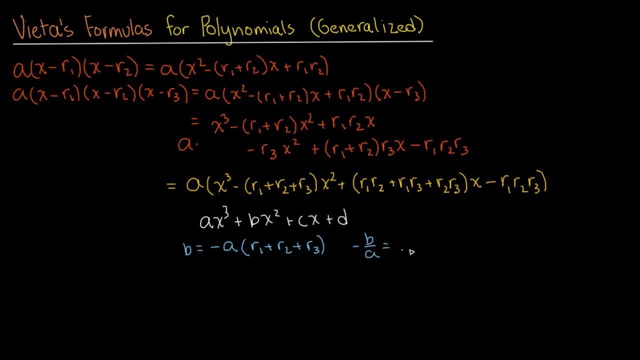 Negative B over A is equal to the sum of the roots. If we, if we look at the constant term first, we see that D is equal to- And we have to remember this- A also Remember this A all the way over here. 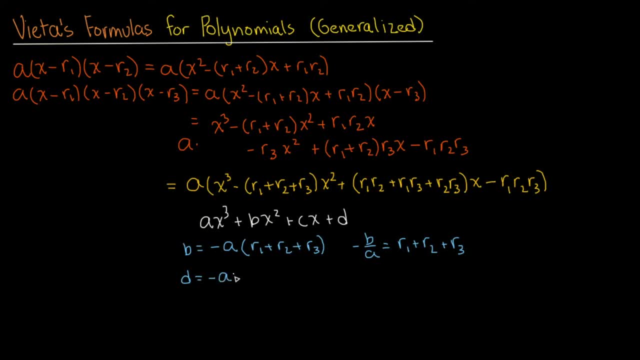 So D is equal to negative A times R1, R2, R3.. So when we divide by negative A on both sides, as before, We see that negative D over A is equal to the product of the roots. Hmm, So there is a difference here. 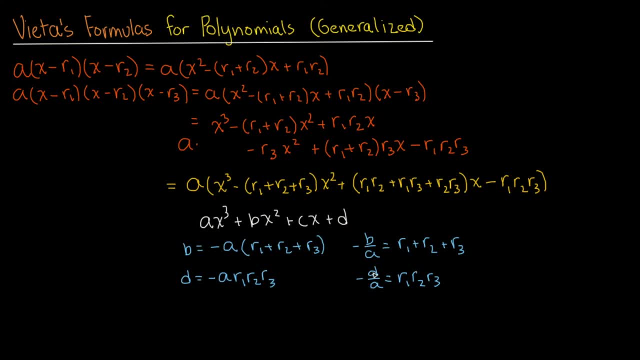 It's not like the negative V over A that stayed the same, But this time, This time, the negative D over A is negative For quadratics. as you may remember, it's it was C over A, not negative C over A. 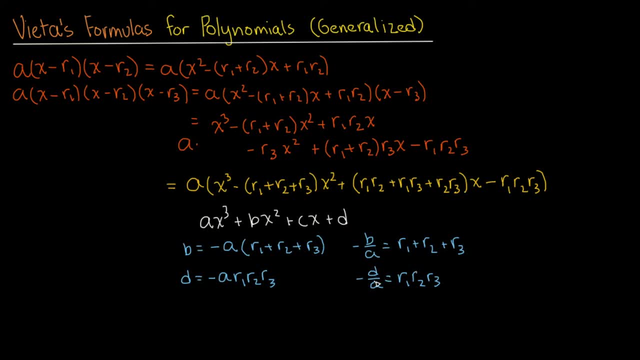 So. so it's interesting to see that it's actually negative D over A here for the product of the roots of a cubic. Well, we do have the the very new thing over here: The R1, R2 plus R1, R3 plus R2, R3.. 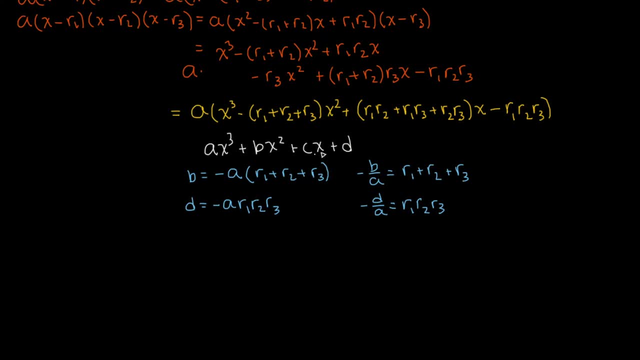 So let's look at that. We see that C is equal to A times this, So I'll write that over here. C is equal to A times R1, R2 plus R1, R3 plus R2, R3.. And when we divide by A on both sides: 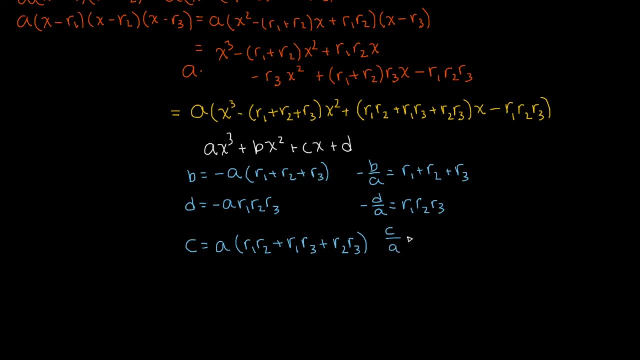 We get that C over A Is equal to R1, R2 plus R1, R3 plus R2, R3.. And this is a new, new formula because we don't see a direct use of this. It's not exactly a sum of the roots. 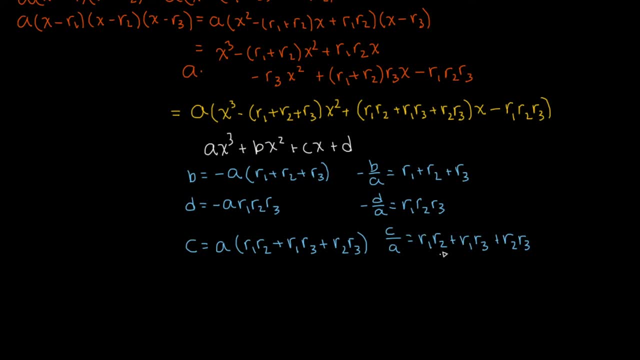 It's not exactly a product of the roots, But What? what exactly is it? Well, we notice that it's the combinations of when we choose two of the roots. Now, why does this make sense? Why would it be that that, for the X term, we run through the combinations of choosing two of the roots? 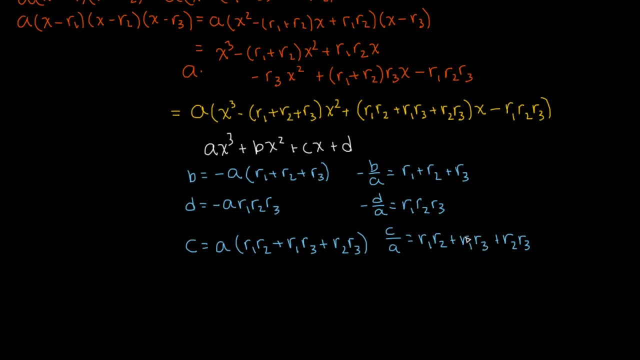 Why? why wouldn't it be three of the roots, for example? or or one of the roots, And we see that in total, actually That this gives us a better picture of what The sum of the roots and the product of the roots actually is. 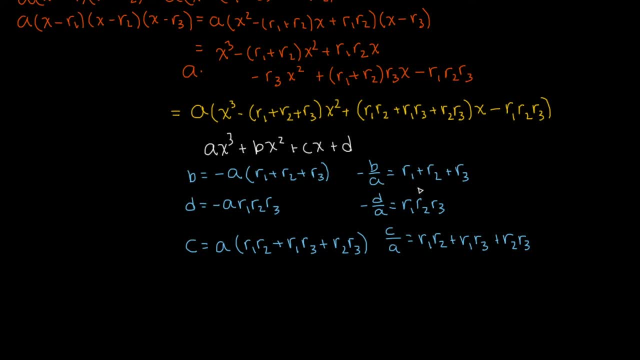 Because the sum of the roots is simply the permutation of the roots when we only choose one of them. Because there's only one way to choose each root, So we have R1 and there's no other. no other R1 to write down. 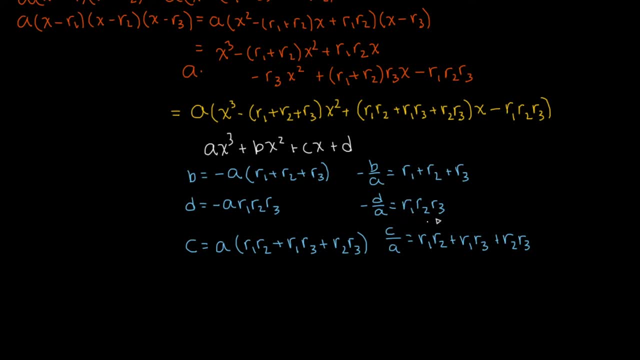 And we have R2 and R3. similarly, And for the product of the roots, It's the way that we can choose three roots And sum them all, But since there's only one way to choose three roots, there'll only be one term in this sum. 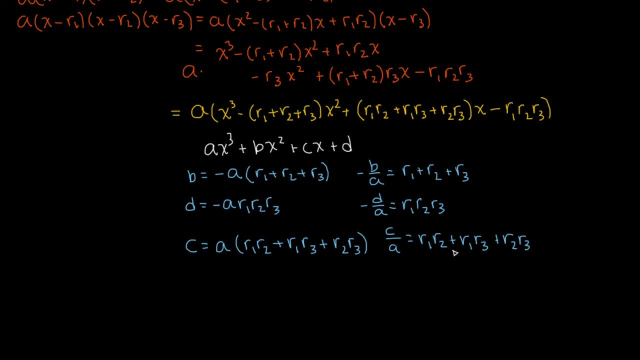 But here we're choosing two of the roots We're choosing. we're choosing either R1 and R2.. We're choosing either R1 and R3. Or R2 and R3. And since we have different combinations of these, we write them all down. 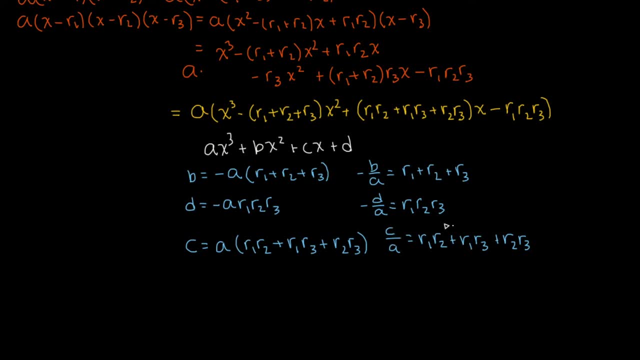 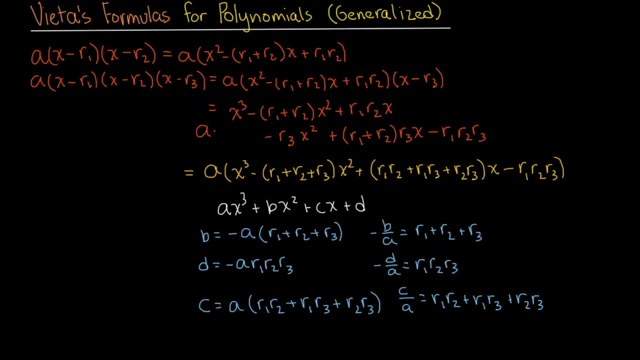 So that is why that is what we observe here, But why does it happen? So let's think about it. think about it intuitively. If we look back over here- and I'll write this down here Now, what we're actually doing here is when we select an X term, 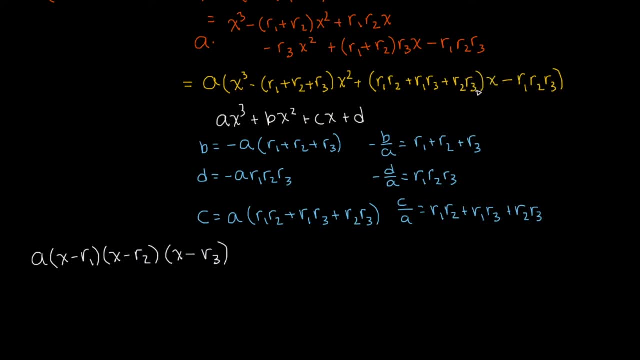 Why would we choose two of the roots? So let's think about that If we choose an X term. So a way we can imagine this is like each of these binomials are boxes With the A on the outside. Each of these. 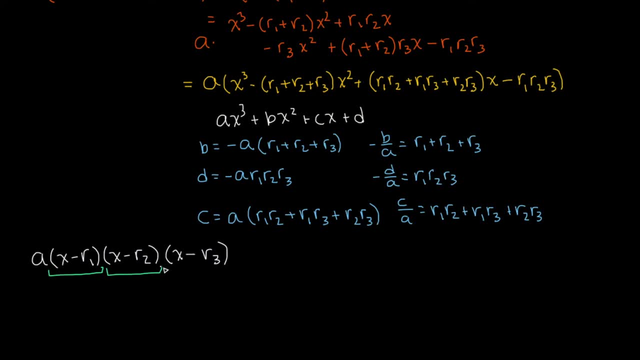 Each of these are boxes And they have two things in them. The boxes have either an X or they have the negative of the root, So you can choose either one of them. So let's say I choose an X out of this one. 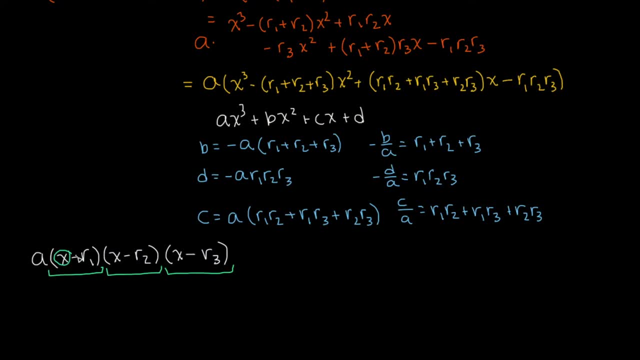 Then, let's say, the rules of the game are: you can only choose one one of those out of the box, Which makes sense because you can't multiply both of them together if they're in the same box. But let's say we choose an X out of this box. 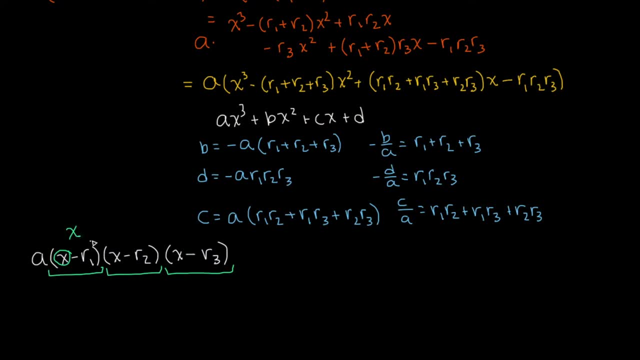 We want to find the X, the coefficient of the X term in the expansion of the polynomial. Well then, since we won't choose any more X's out of these boxes, we'll choose negative R2, and we'll choose negative R3.. 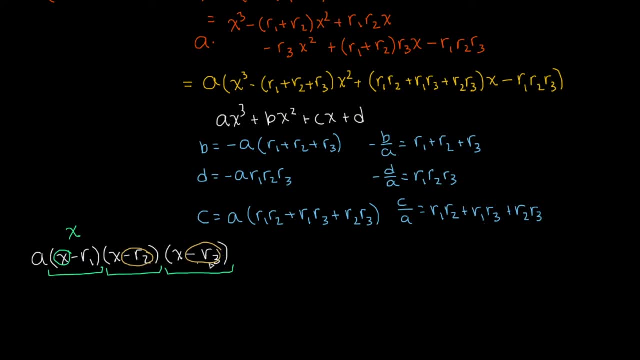 So that's actually what we see over here. When we multiply negative R2 times negative R3, that's positive R2, R3, which is one of our terms over here. So how do we get the rest of the terms? Well, there's three ways to choose an X. 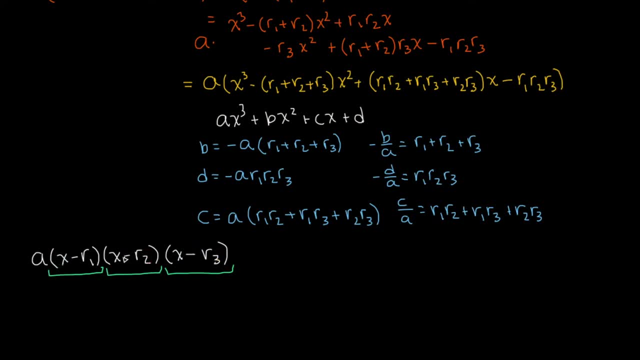 So instead, let's say we chose the X here. So if we chose this X, then now we would choose this R1, and this R3. And, as we see, negative R1 times negative R3 is what we have over here. 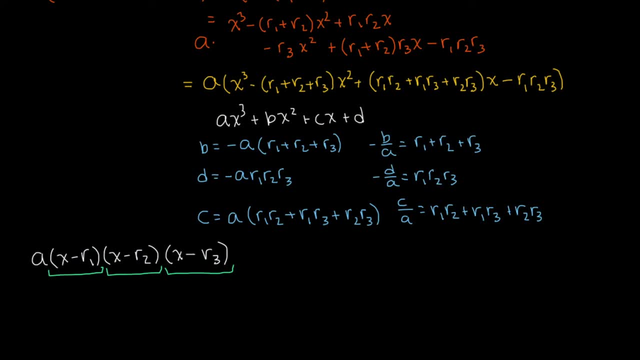 So finally, we just go through the last one. If we choose the X out of here, then of course we have negative R1 times negative R2, which we can see over here. So we can see that all three of these terms that we have over here. 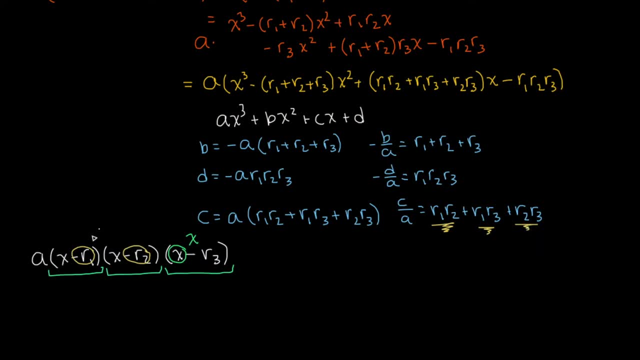 are just combinations of the ways we can choose one X value and two roots. So that's the general idea that we should remember here. We just imagine each of these binomials as boxes and each of these have two items: one X and one root. 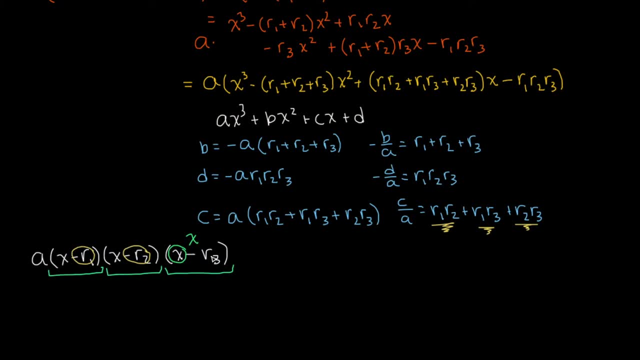 The X's are all the same, but the roots are all distinct. But the basic thing to remember is that when we choose one value out of here, then the rest of what we're choosing is dependent on how many we want to choose. So what we're actually going to do here is see. 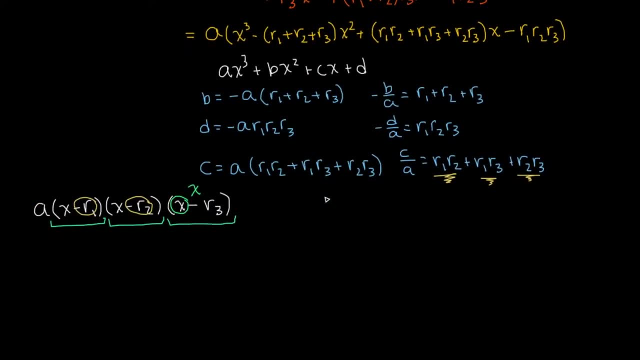 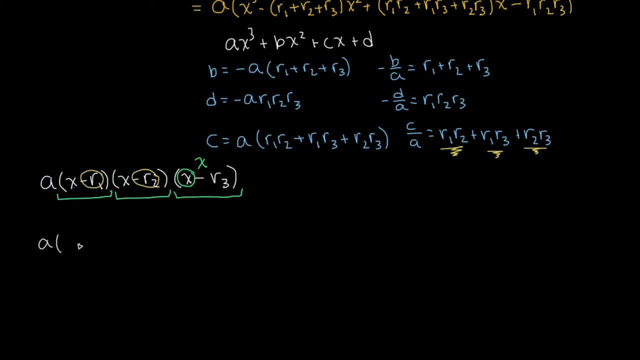 what happens when we look at an even larger degree polynomial. So let's look at A times X minus R1, times X minus R2 and times X minus R3. And instead of expanding it- and we'll of course, add an extra one- 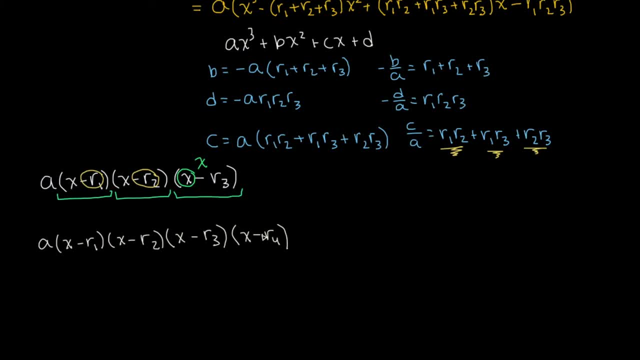 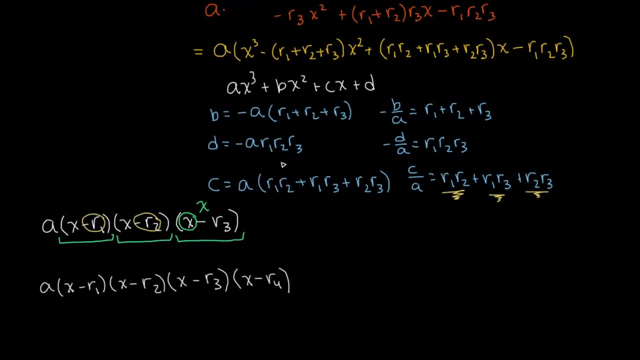 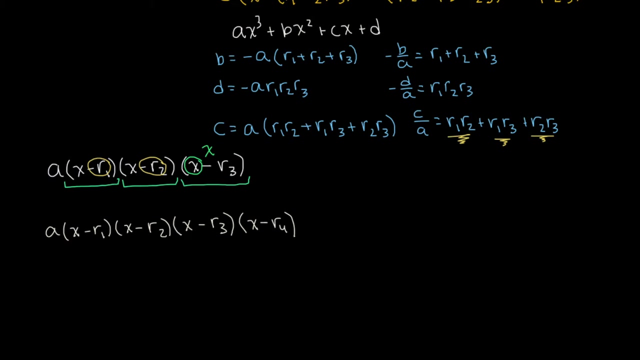 X minus R4, and instead of expanding it this time we'll try to expand it without doing our distribution method that we've been doing so far. We'll try to expand this polynomial using Vieta's formula In this manner. So let's look at that. 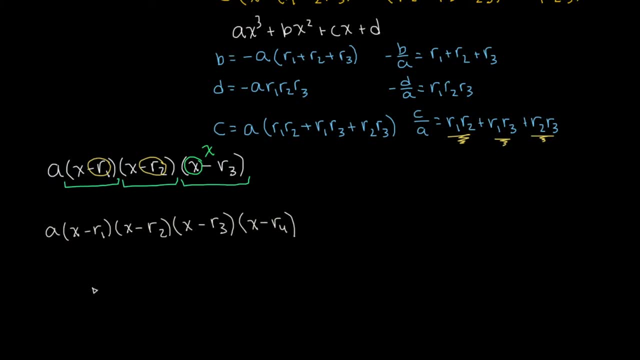 The first term in our polynomial is definitely going to be. In fact I'll write this standard form over here in A, B, C, D, E style, But let's see how we can form this polynomial based on the roots. So first we'll want an X to the fourth term. 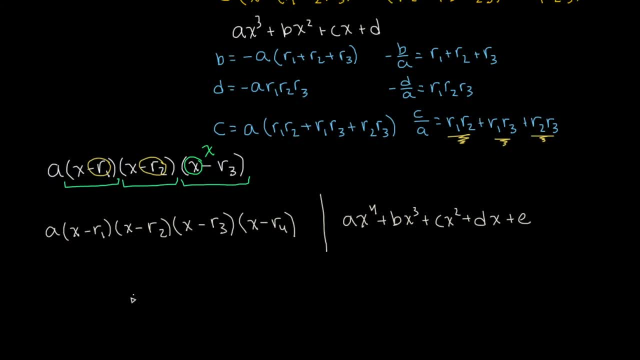 So let's write down the X to the fourth term over here, And we don't exactly know the coefficient yet, But let's see So, and for the purposes of this, I'll keep the A on the outside, just because it's easier to see the patterns that are going on here. 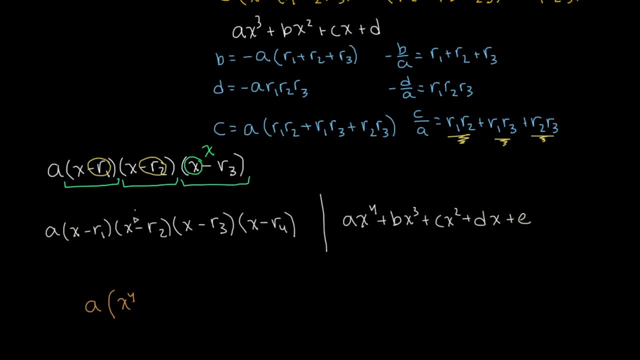 So we have an X to the fourth. which? how many ways can we write the coefficient of X to the fourth? Well, in order to get four X's from each of these boxes, we have to choose one X, Since we've already chosen from the four boxes. 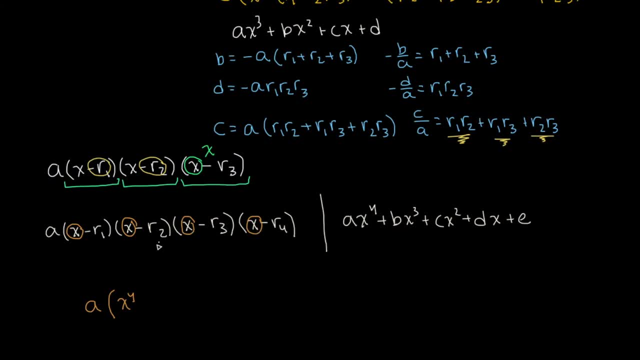 there's no more coefficients that we could get. There's only one possible way to choose four X's when there are four boxes. So this will be our only One, will be our only coefficient for the X to the fourth term. So if we look at the X to the third term, 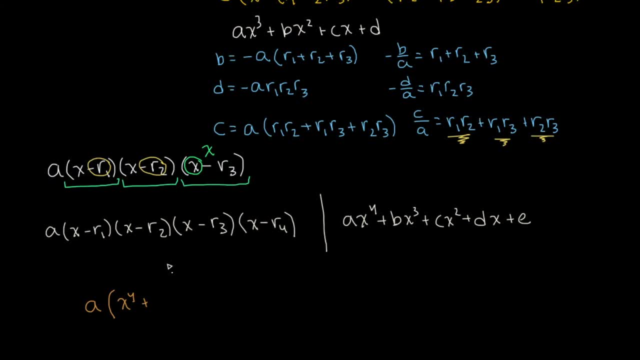 and I won't write anything yet because there might be other ones. Well, let's see, So we have X, We want to choose three X's, So we'll choose three Like, so We'll choose from each of the three boxes. 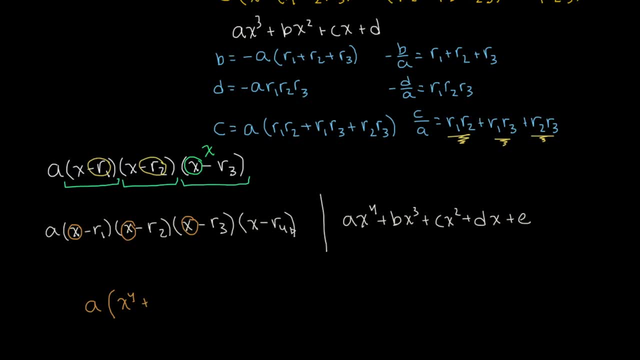 And, as you can see, we only have one. We only have one root left to select, And this will happen every time. There's only When you choose three X's, there's only one root, One root left remaining to choose from. 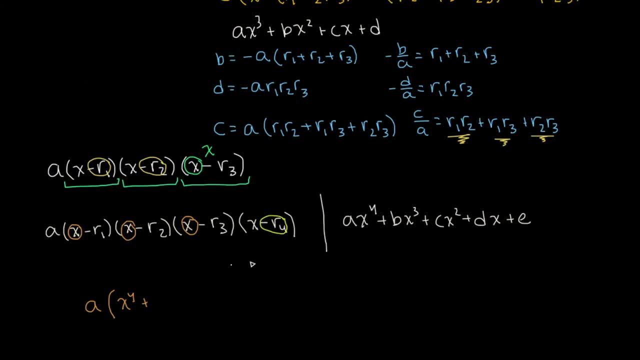 So the coefficient in this case will be the sum of the roots. But how will you tell whether it's a negative or positive? The way to do that is simply check the number of roots that you are permuting, So the number of roots that you are running through. 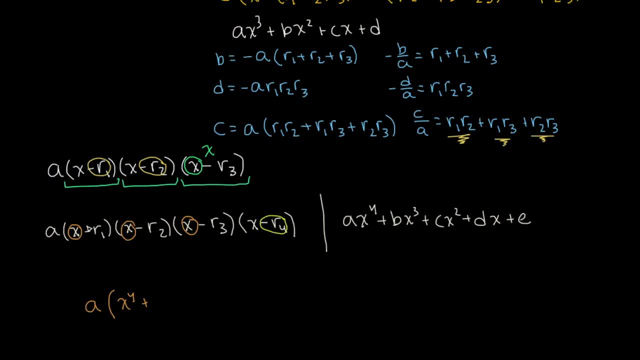 So since we're only running through one root each time, a negative will stay Like negative one, So I'll actually write that down. We know that negative one, The power of any odd number n, is equal to negative one. So the same idea. 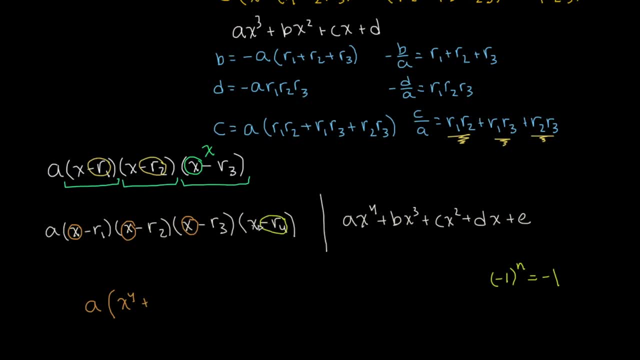 when you're only choosing one root, or if you're choosing three roots, negative one to the power of one or negative one to the power of three would still remain negative one In that idea when we have, When we're choosing one root. 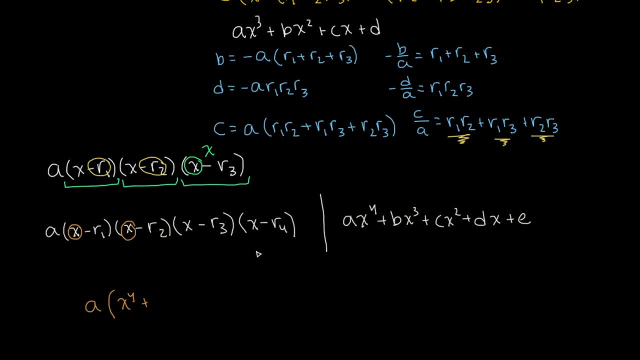 we know that this must actually be negative. So let's actually change that. So this will be negative. And of course, we realize that, since we're only choosing one root at a time, this would be the sum of the roots. 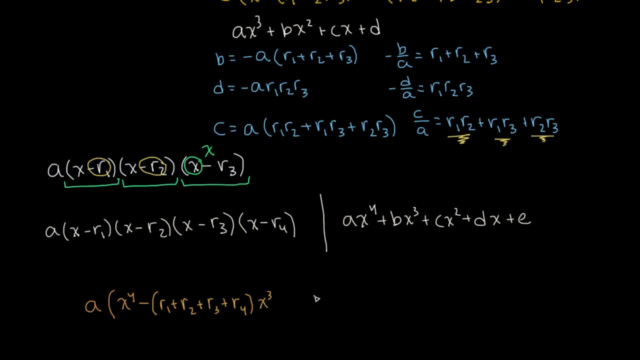 But that'll be our x to the third term. So that's very interesting, And since we already got an odd power here, we know that the next one is going to be positive. Since it alternates, it's like you got a. 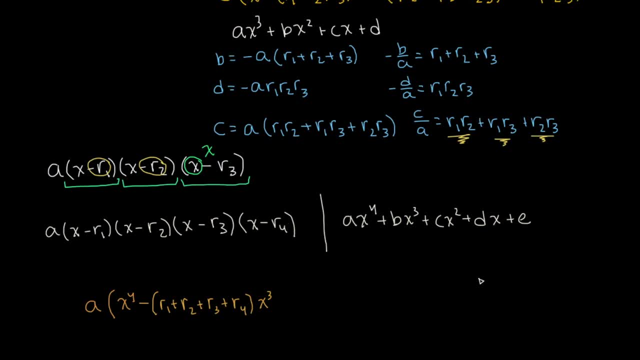 Negative one to the power of one is negative one, but negative one squared is one, So we'll have a positive here. We already know So what happens when we choose, When we choose two x terms. So let's choose two x terms this time. 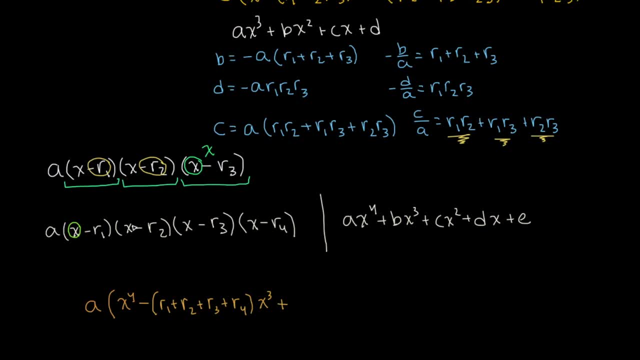 So if we choose two x terms, then we have two over here, And we see that we have. We have two roots left to choose from. We have the negative r cubed and the negative r to the fourth. We have both of these roots to choose from. 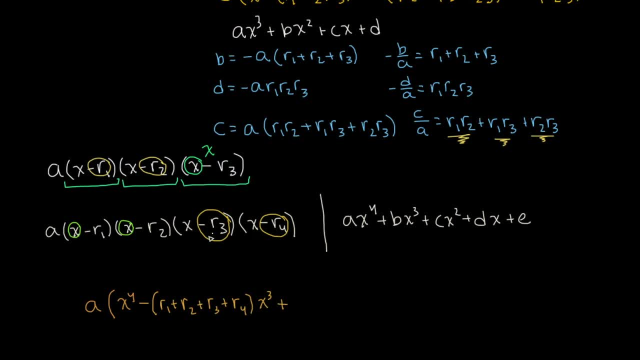 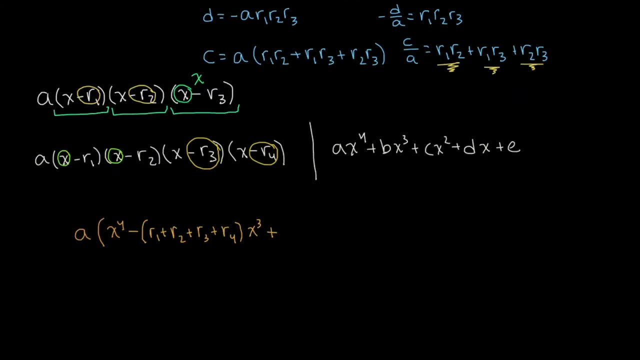 So now we're running through two of the roots, So all we have to do is go through all the permutations of two of the roots, However we. However, we don't want to repeat any, So the way we'll do that is by: 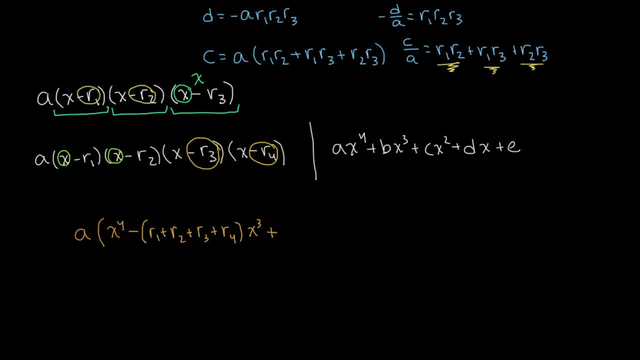 by listing them out and and figuring out if we have repeated any. So let me first remove these and we'll write them down. So first we have. If we choose from the r ones, Let's say one of ours will be r1. 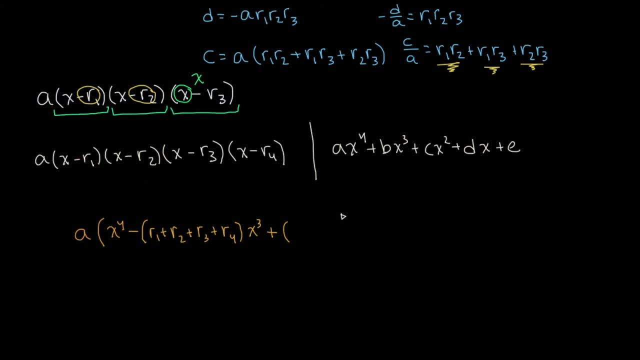 We want to choose an r1 from this box, So we'll have an r1, r2.. And remember, this is all on the basis that we're choosing two from this, So r1, r2.. r1, r3. 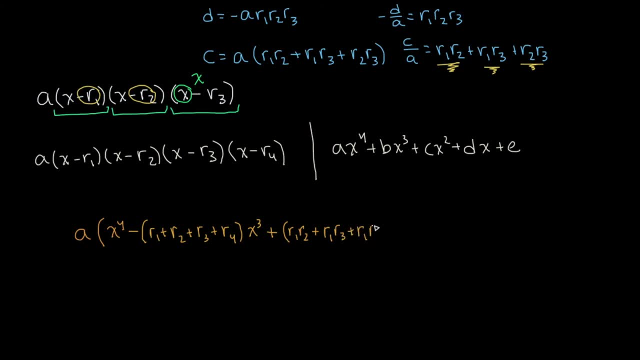 plus r1, r4.. And that's all of the things we can do with r1.. So now let's go to r2.. But we, Since we We can't exactly do r2, r1 because we already did r1, r2.. 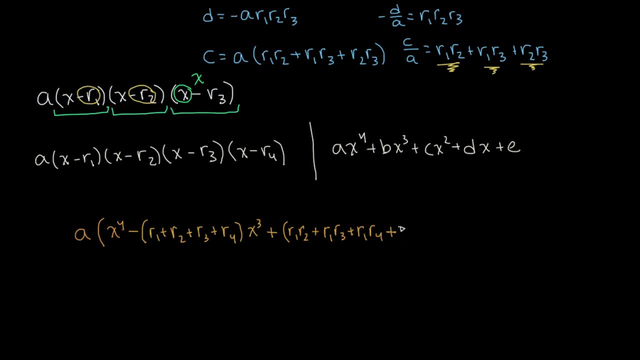 So we'll just go to the right again: r2, r3.. plus r2, r3.. and then plus r2, r4.. With r3, we already did r3, r2 and r3, r1.. 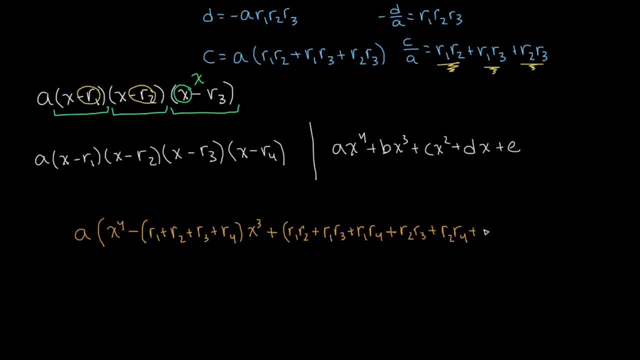 So we can only go to the right again, which is r3, r4.. We've already done everything with the r4. We can't go to the right anymore, So we'll close it off And that will be the x squared coefficient. 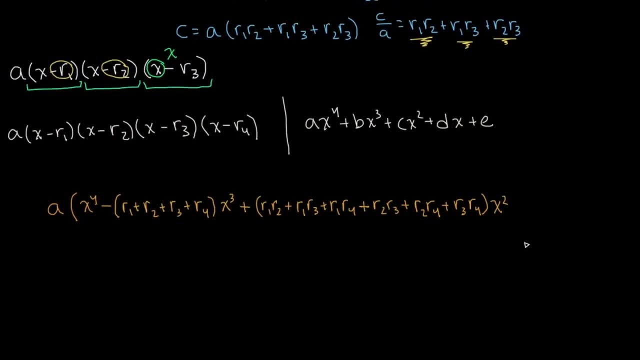 Now this is starting to get interesting. So now we have our x coefficient. Now we're running out of space here. But with the x coefficient what we're doing is we're running through cycles of three roots, because when we choose an x over here, 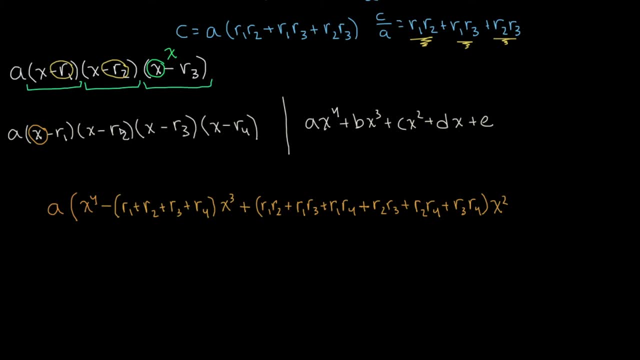 what we have left? what we have left is that we're choosing three of the remaining roots. So we're choosing negative r2, negative r3, negative r4.. Now, since we're choosing an odd number of roots, we know that from our experimentation. 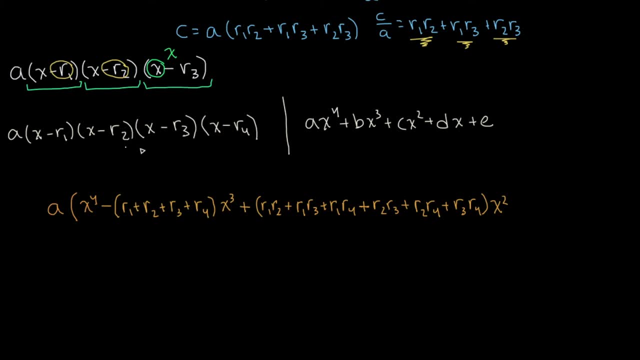 and logical thinking we have, and we have a negative term, So I'll actually write this over here. We're going to run in cycles of three. Well, we know that we'll have a total of four permutations of three, Because there's only one way to choose. 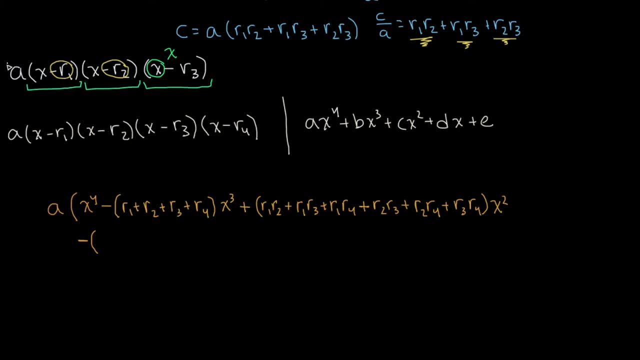 there's four ways to choose one x out of each of these boxes. We can either choose here. we can either choose here, here or here. So we'll know we have four, So let's keep that in mind. So we have a negative times: r1, r2, r3.. 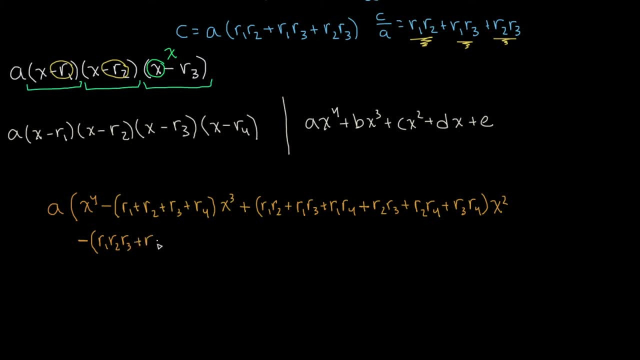 That's one of them. We can also do r1, r2, r3.. r4.. So that's one of them. Now we can also do r1, r3, r4.. And the last one we didn't do is r2, r3, r4.. 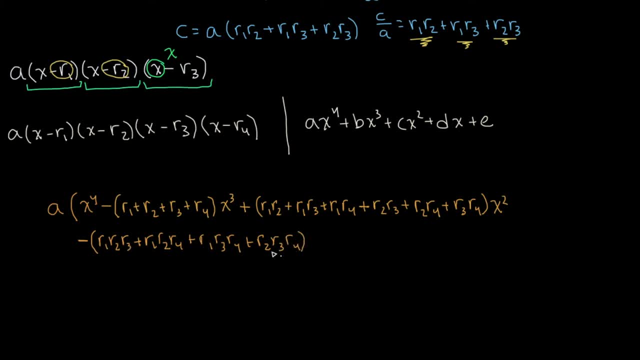 And we can be confident that we ran through all of them, as long as none of them repeat, because there's only four ways to choose one x, Or there's only four ways to choose three roots. So as long as none of these repeated. 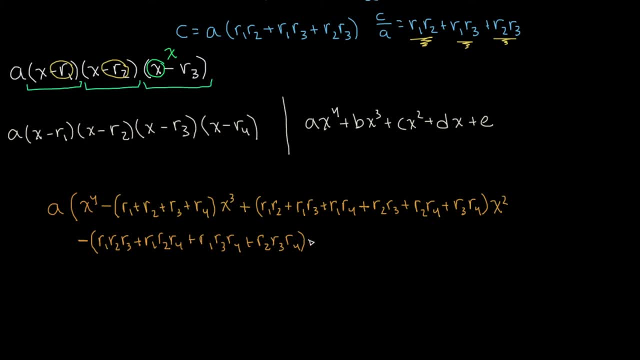 which you can see that they haven't. we can close that off And that'll be our x term. And now, finally, we have our constant term, which we can be happy about seeing, because that is simply choosing four of the roots. 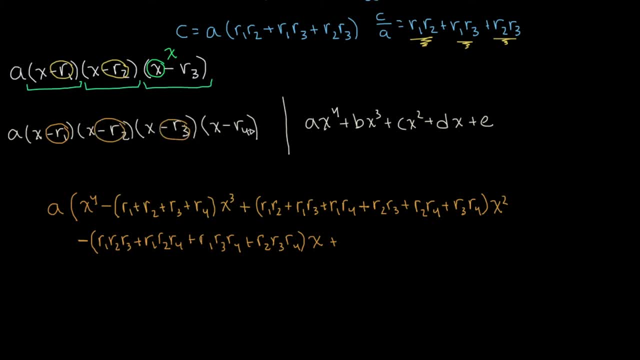 which, as we can see, there's only one way to do, And it's even even number of roots, so we can add them: r1, r2, r3, r4.. And this is how. this is Vieta's formulas. 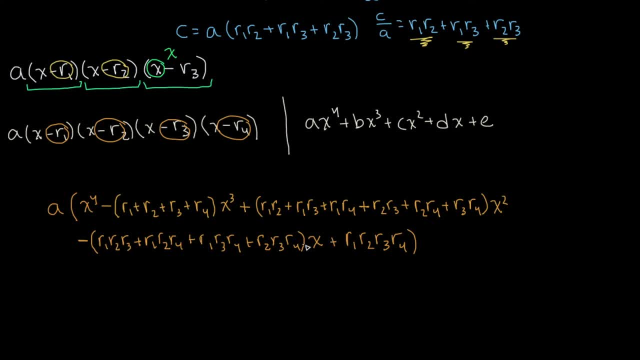 for the general, any general polynomial, And you can see, like, let's say, I gave you a, let's say I gave you a six degree polynomial and I asked you: well, hey, what is the coefficient of the x squared term? 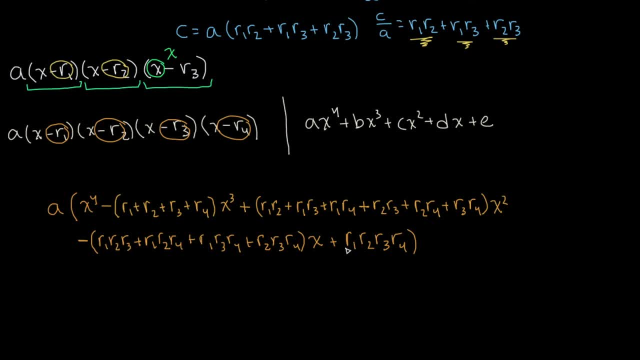 Of the six degree polynomial in terms of the roots, Using this box method, or if you're familiar with familiar with combinations, then that might just be easier for you to visualize. But you could tell me, based on this Vieta's formulas idea. 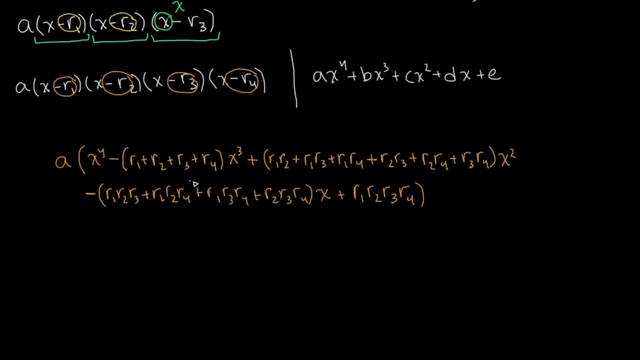 So, to finish it off, let's just write down the formulas that we have in terms of these coefficients. So let's say we have the sum of the roots of this polynomial Is, and I'll just make it. I'll just make it over here. 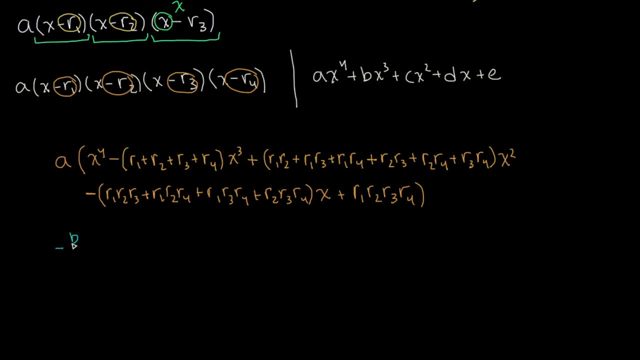 So we have the sum of the roots of the fourth degree polynomial is negative b over a And that is equal to r1 plus r2 plus r3 plus r4. And we have the- actually I don't know what to call it. 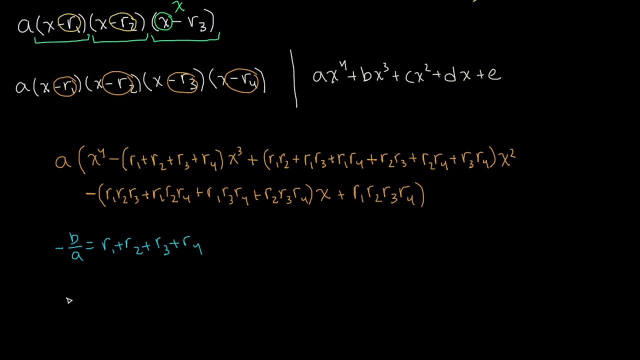 but we have this, which is equal to, which is equal to c over a, And that is equal to this. And now an easier way to write this is actually just. this is a symmetric sum, or this is what is known as an elementary symmetric sum. 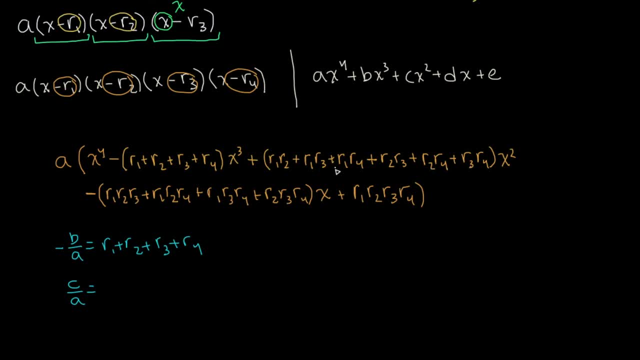 And that basically means that we're running through the permutations of these, of these values at a, at a, at the basic level. So I will call that s of 2, as it's the second symmetric sum that we see here And we see that. 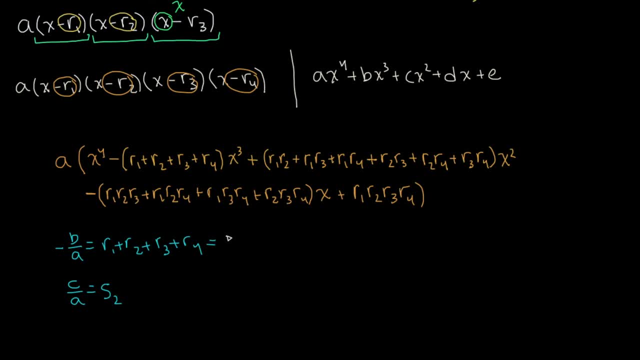 so this, this you can also write as s of 1.. And then we have negative d over a, which is equal to the third symmetric sum. And finally, we have e over a, And that is equal to the fourth symmetric sum. 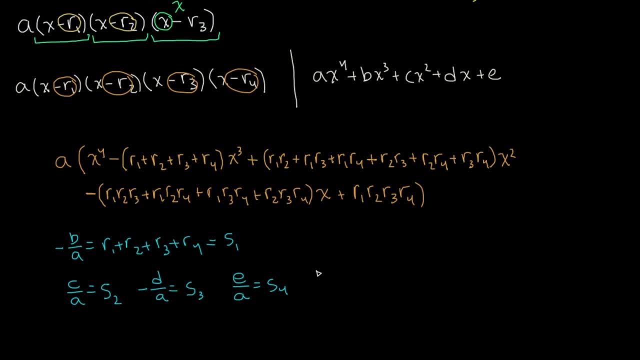 Now- hopefully this was interesting- How we could figure out that polynomials, if we change our perspective a little, you can actually think of them from a combination perspective, or these, these interesting patterns of the symmetric sums, And that that really changes our view on polynomials.